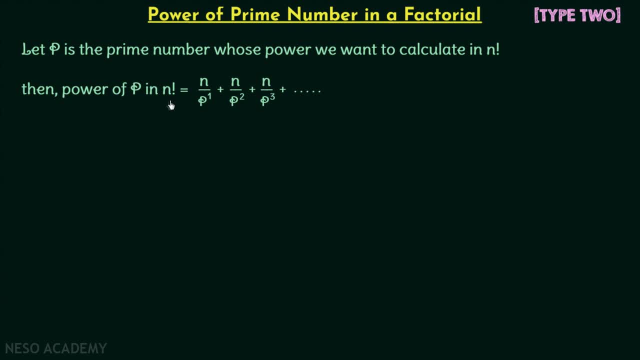 highest power of prime number p in n factorial. Now, regarding this formula, there are two important points. The first point is: after the division take only the integer part. This means when you perform the division, then after the division take the integer part and then do the addition. For example, if n is, 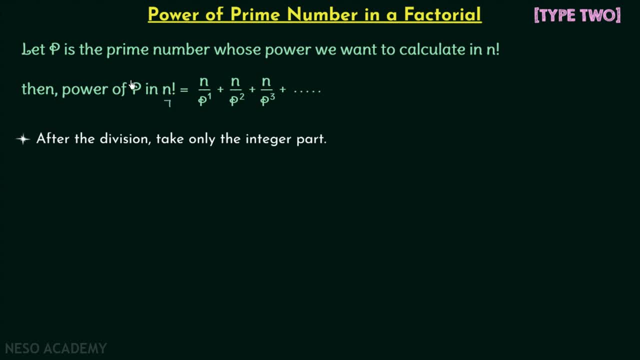 equal to 7, we will have 7 factorial. and if p is equal to prime number 2, then we need to find the highest power of 2.. So the first point is the fact that we need to find the highest power of 2 in 7 factorial. 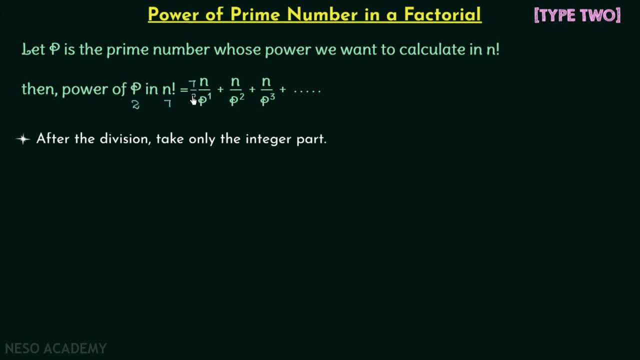 Then, focusing on the first term, we will have 7 divided by 2, power 1, which is 2.. So, 7 divided by 2, we will have 3.5.. Now here we have two parts: 3 is the integer part and 5 is the. 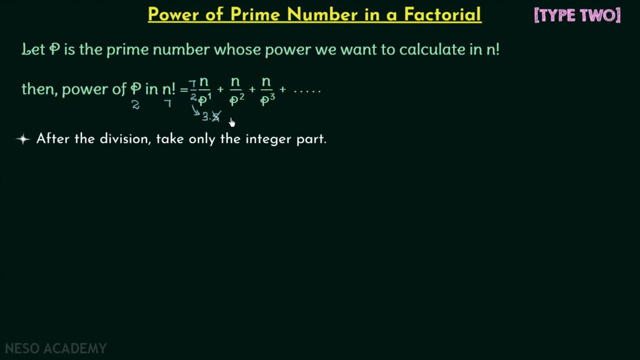 decimal part. We need to take the integer part, that is 3, and we need to reject the decimal part, which is 0.5.. we will follow after performing the rest of the divisions. So I hope point number one is clear. Let us now move on to point number two. Ignore the term and the 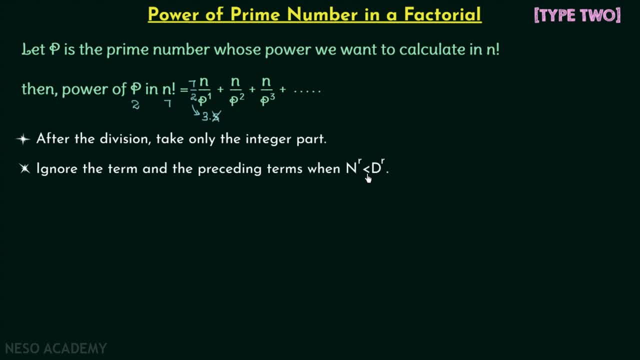 preceding terms when the numerator is less than the denominator. Now, this point is an important point and this point we have obtained from the first point itself. According to this point, when the numerator is less than the denominator, we can ignore that term and the preceding terms. Let us try to understand. 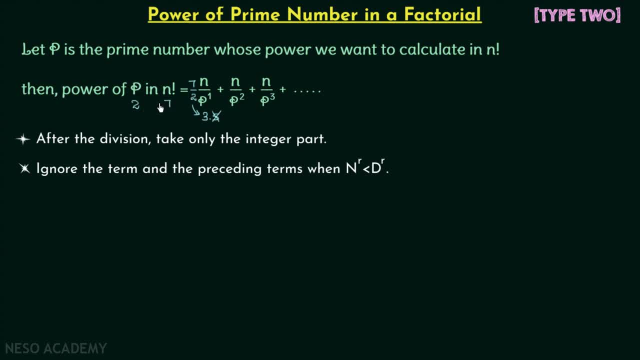 the reason for this. We will take the same scenario: n is equal to 7 and p is equal to 2.. Now focus on this term: n over p, cube n is 7, p is 2.. So we have 2 power 3. 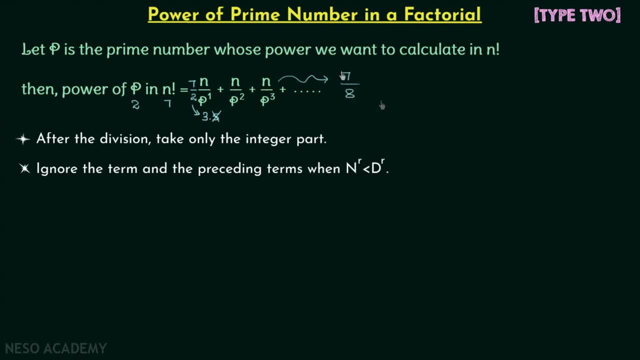 and 2, power 3 is equal to 8.. The numerator is 7, the denominator is 8, numerator is less than the denominator and numerator is less than the denominator, less than the denominator, and from here, when you perform the division, you will have 0.875.. 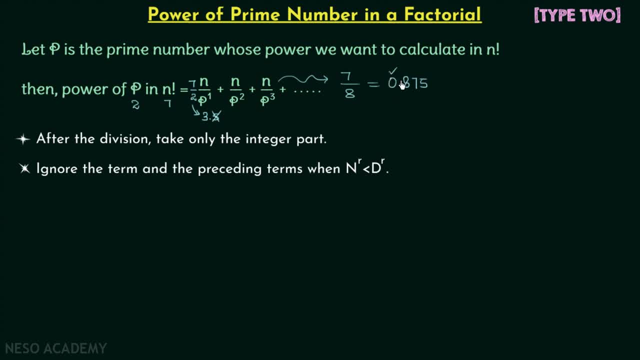 And, as per our rule number one, we will select the integer part and we will reject the decimal part. So we are getting zero from this term and adding zero to these two terms. the result is not going to get affected. And when you consider the next term, which is n over p power, four, again you are going. 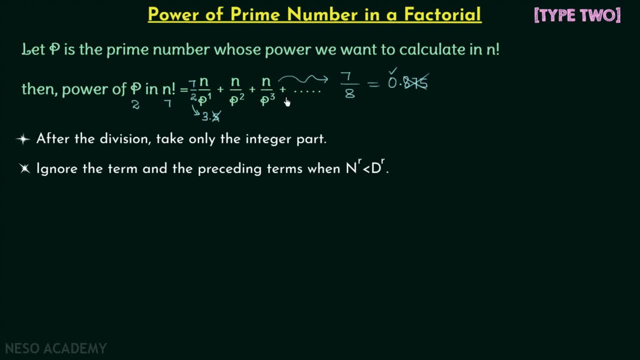 to have the integer part equal to zero. So we can say that whenever the numerator is less than the denominator, the integer part is going to be zero from rule number one, and that is why we can neglect that particular term and the preceding terms. So this is what we mean by point number two. 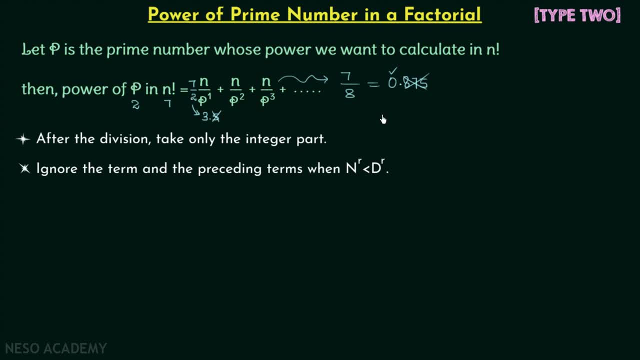 So in this way we are done with understanding the formula, and now we will move on to our problem, Problem number one. In this problem we need to find the power of two n, four, factorial. So here, two is our prime number, p, and four is our number n, and the power of two n four. 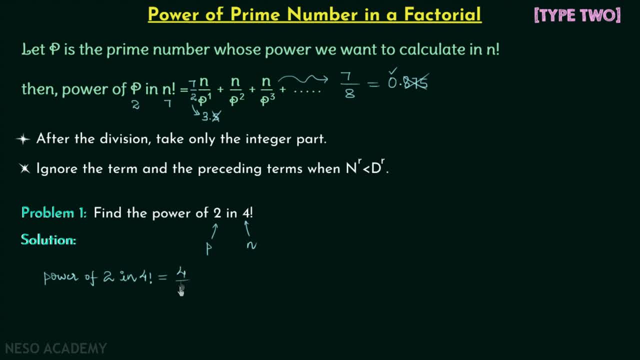 factorial will be equal to four divided by two power one plus four divided by two power two. Two power two is equal to four. Numerator and denominator: both are same. We will consider two. We will consider the next term. four divided by two power three. 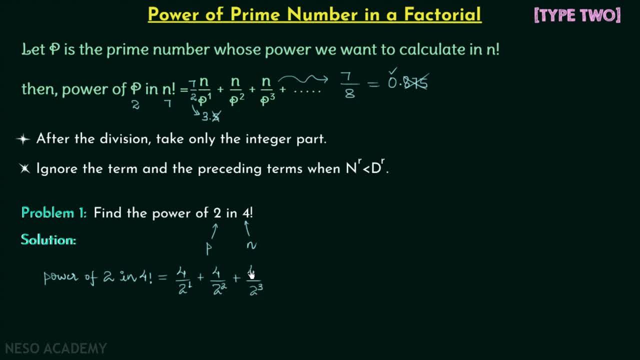 Two power three is equal to eight. The denominator is larger than the numerator, So we will stop here Now, moving on to the calculation part. Four, when divided by two, will give us two. Four when divided by four, will give us one. Four when divided by eight, will give us the integer part equal to zero. 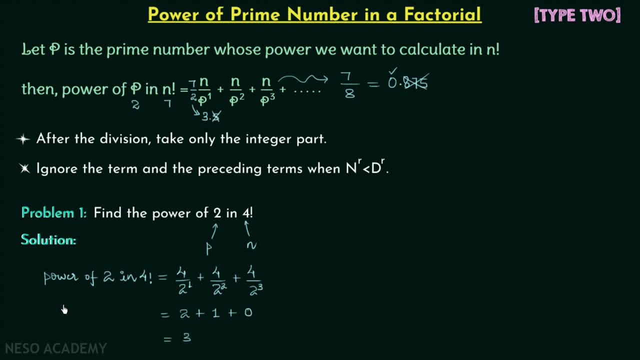 So we have three as the answer. So the power of two, which is The highest power, Don't forget this, This is the highest power of two in four. factorial is equal to three. Now, moving on to our problem number two, we need to find the power which is the highest. 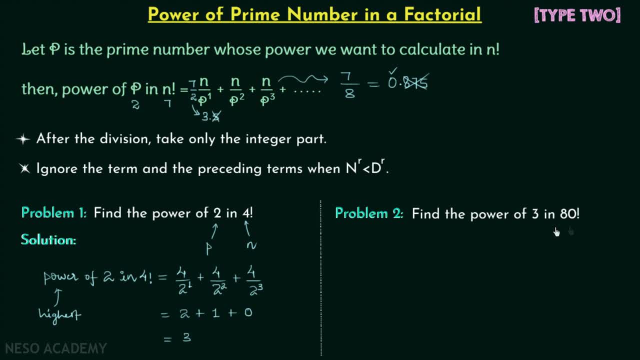 power of three in eighty factorial. So in this case our prime number is three and number n is equal to eighty. We will find out the highest power of prime number, three In eighty factorial. This will be equal to eighty divided by three power one.